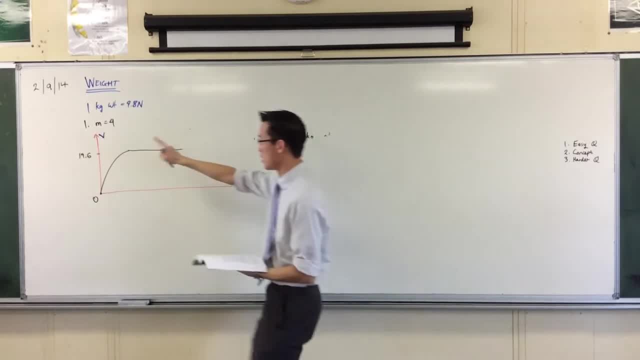 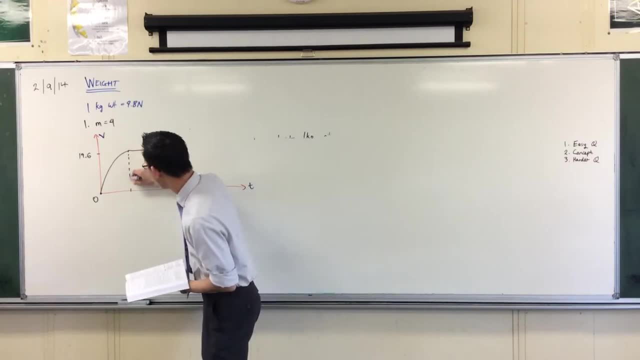 Remember, this is not a displacement graph, This is not displacement time, This is velocity. The thing is moving, but the velocity isn't changing. Okay, So at some time- which I don't know what it is- it stops. the force stops acting, right. 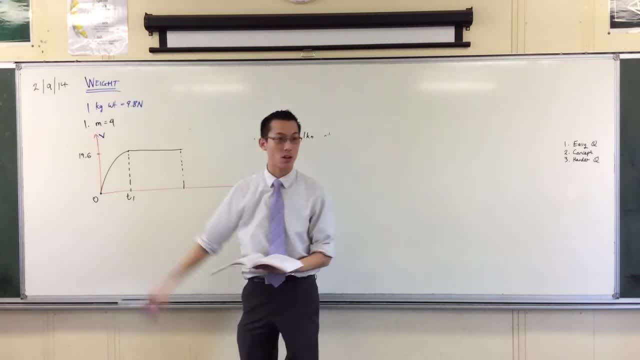 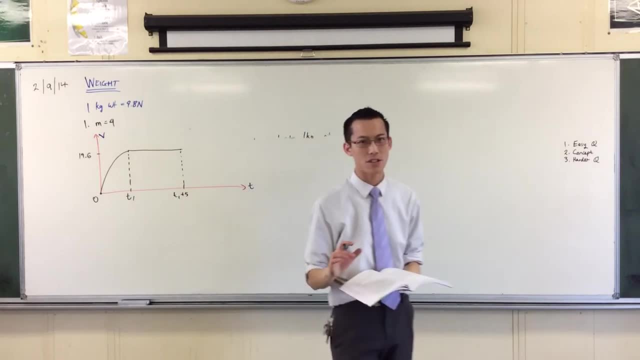 And then for 5 seconds it moves at this constant rate. It moves at this constant rate, right? So, whatever this time is, after 5 seconds. that's when the behaviour changes again. for the final time. It's then brought to rest. 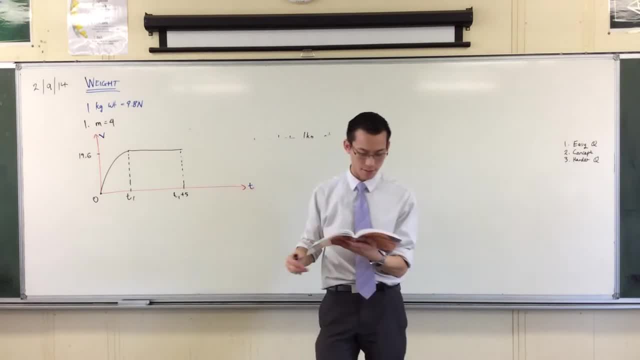 So it's going to. this is going to come back there. It's brought to rest by a constant force of 5 kilograms weight Brought to rest. So it's going to come down at a constant rate, right? Something like this. 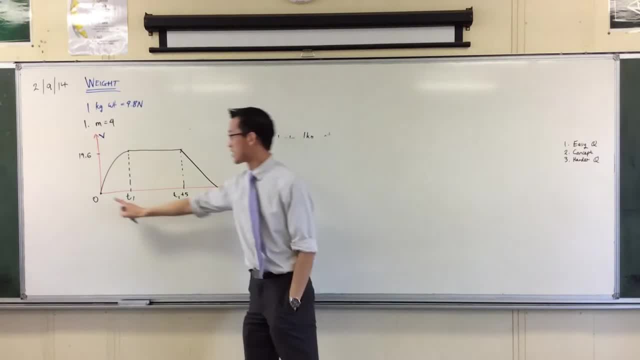 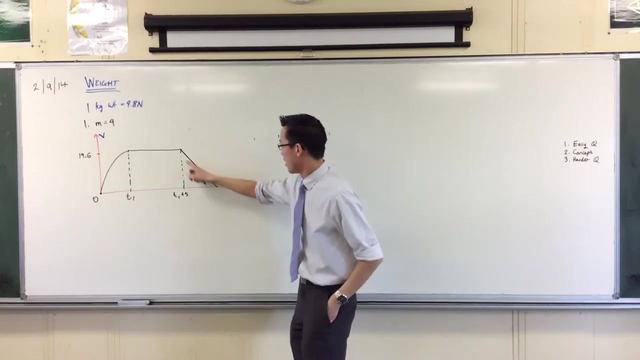 Okay, there you go, I'm finished right, Start from zero. a force starts acting, it gets to a certain speed. force stops, 5 seconds elapse. Then a new force- totally separate, you can see the equations are completely different- acts on it and brings it back to rest. 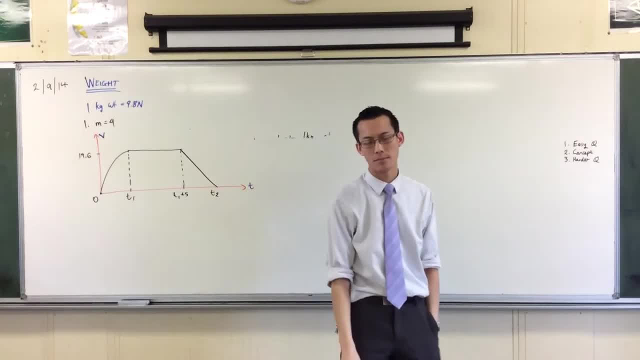 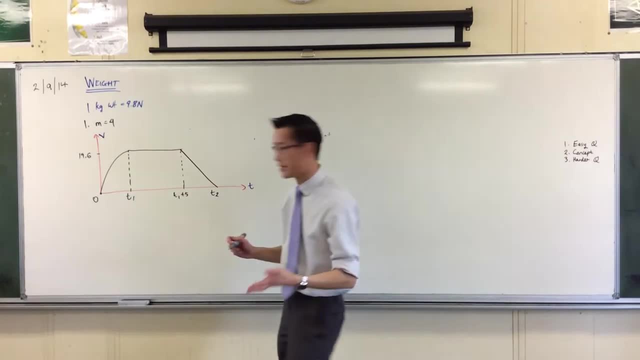 I don't know when it rests, but it'll be some time that I'll need to work out later on. Okay, So you can see here I have a piecewise function right. To make it a bit easier for me, I'm going to name these different sections. 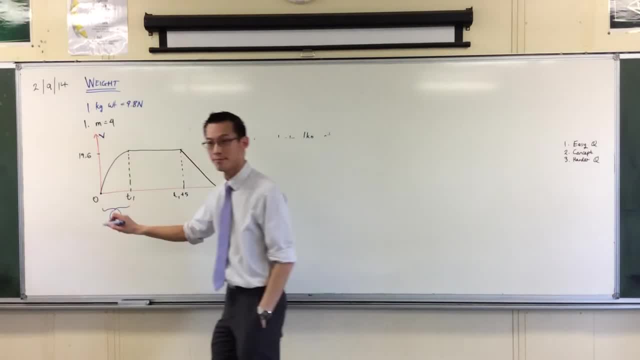 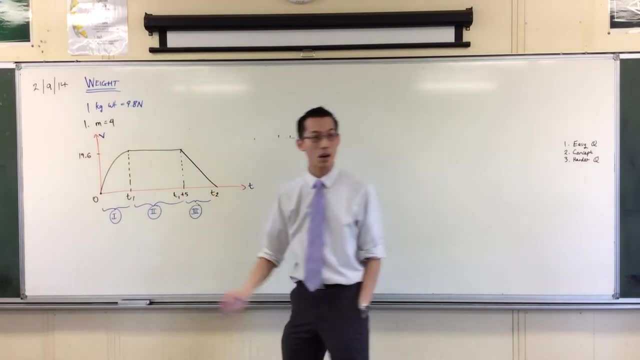 Okay, So I'll call this one Section 1.. This one is Section 2.. And then I have my last, Section 3.. Okay, Let's take them one at a time. How far does he go? That's the question, right. 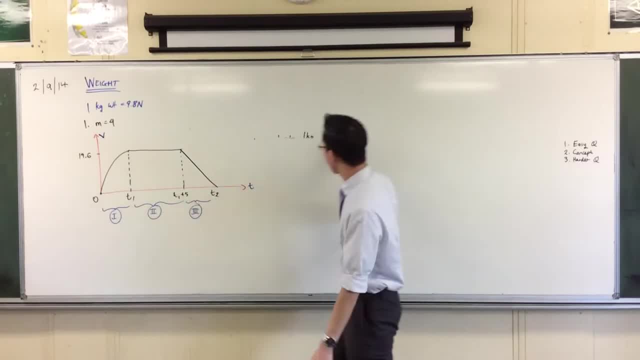 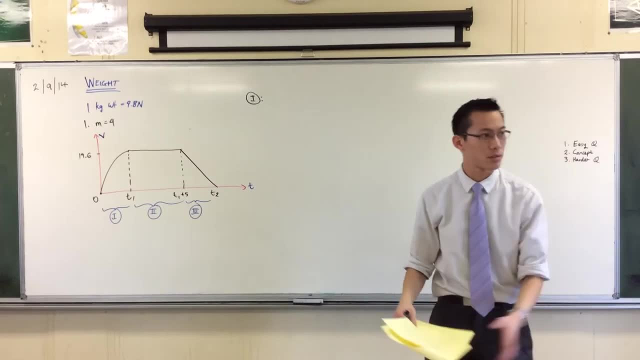 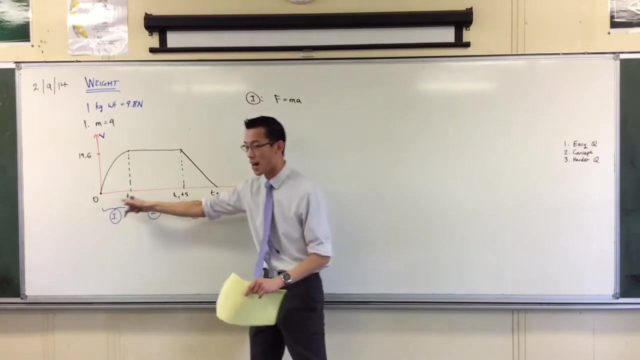 So let's have a look at the first portion Now. we start with force right, Because they give us an equation for force. So I've got force equals, ma right Now, for this part of it, they give us a force equation. 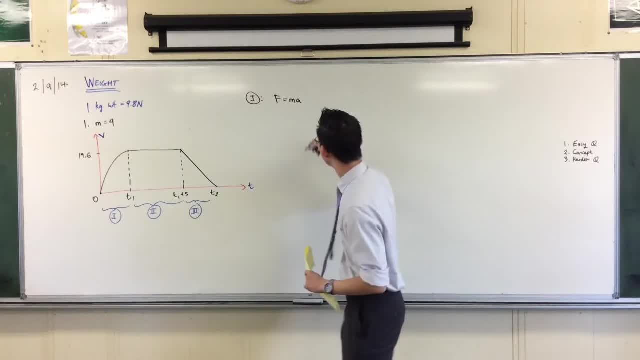 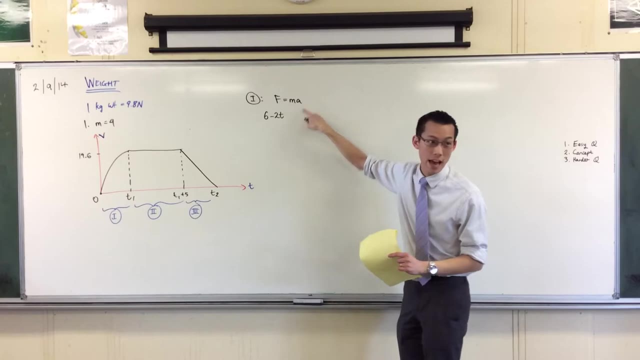 They say it's 6 minus 2t Kilograms weight. Now stop. Kilograms weight Mass, that's kilograms. Acceleration, that's meters per second squared. So this side of the equation, the ma side, it's in newtons, right. 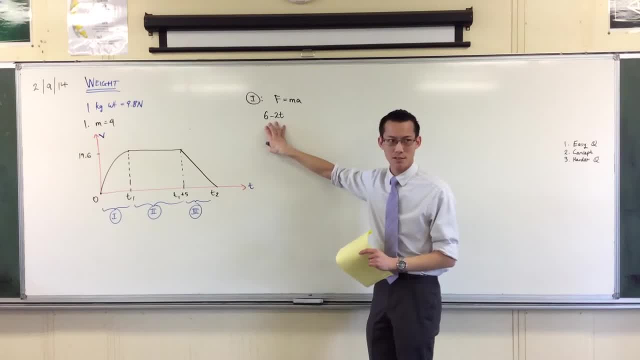 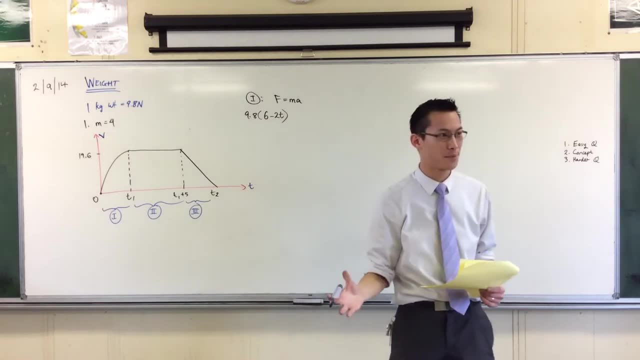 But then this is not in newtons, right? It's not in newtons. In fact, it's in kilograms, weight which is 9.8 times bigger than newtons. Okay, So I've got this scale happening, Okay. 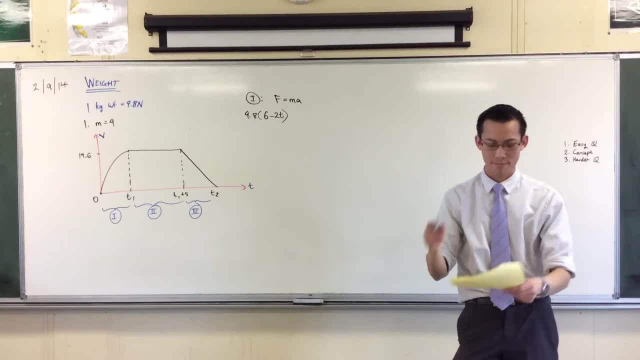 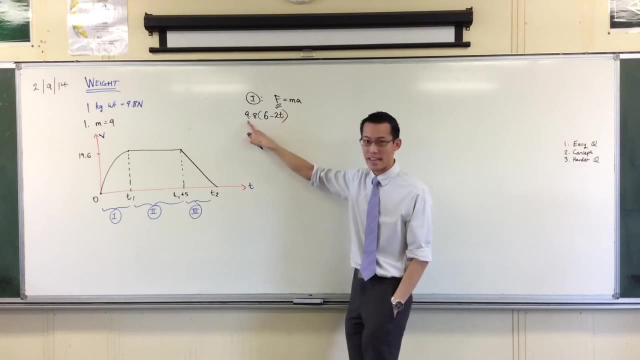 Is that alright? Let's think about this. The force right. The force is 6 minus 2t kilograms weight, So that's why it's bigger. I need to get- This is in newtons- right. This side is in newtons. 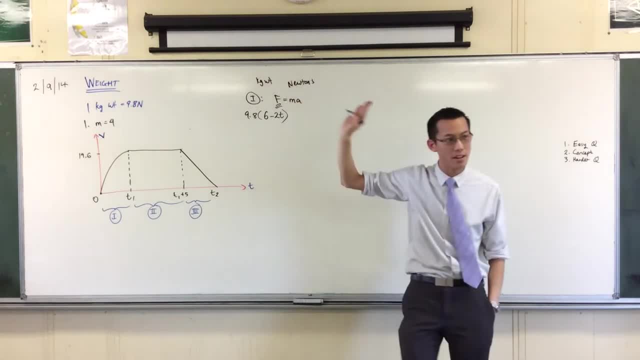 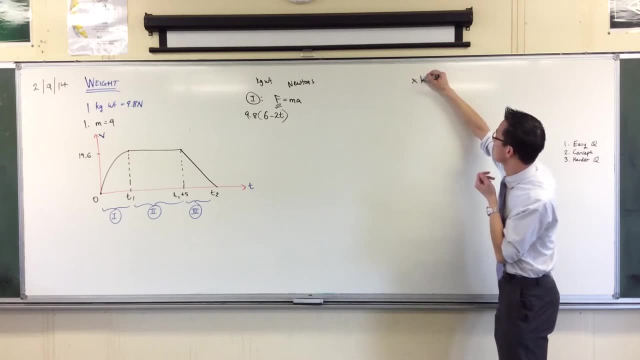 And this side is in kilograms weight. But I don't want them to be different, okay. So, if you like, if I said, for instance, you've got like x, let's see kilograms, Just think of weights, okay. 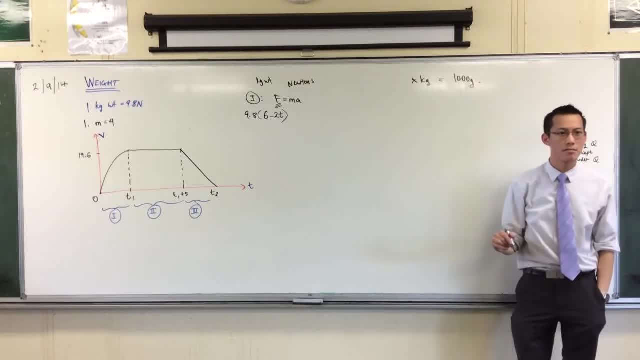 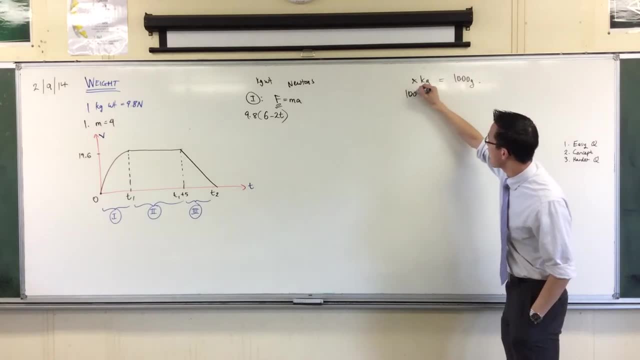 Equals 1,000 grams, right? So, in fact, what's x? in this case It's 1, right, Because it's 1,000 x grams. Okay, So I've got tiny, tiny units over here and big units over here. 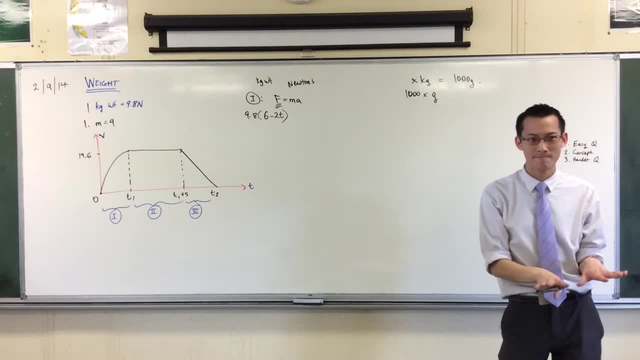 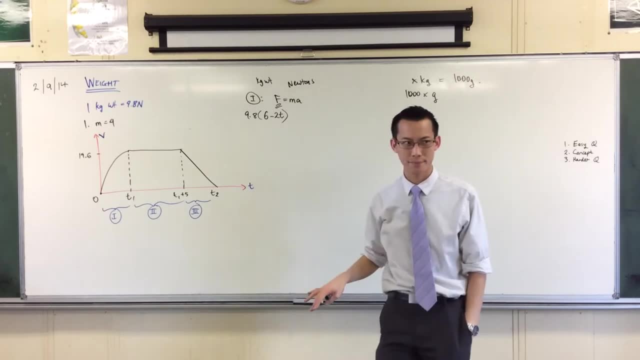 So that's why I multiply to compensate. Okay, So kilograms weight are bigger than newtons. They're 9.8 times bigger. Okay, So that's where it's going to go, Is that okay? Good, Alright. 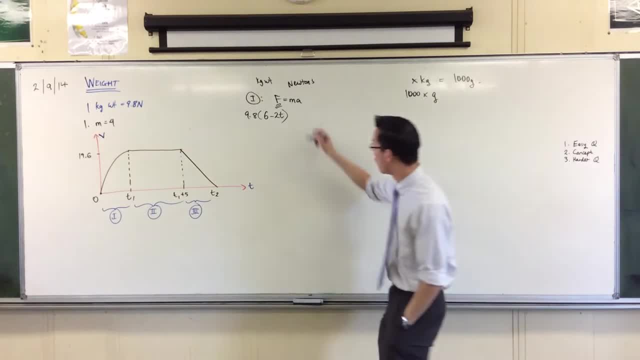 Then I have a mass of 4 and I don't know what acceleration is. Okay, But that's okay. I can rearrange this thing. Let's divide. Let's see here: If I divide this by 2 and then I divide this by 2, I'll have divided by 4.. 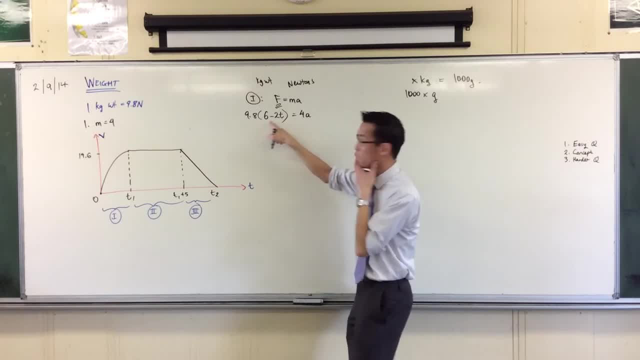 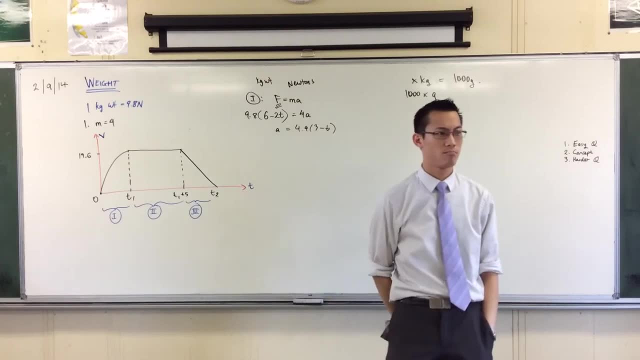 Is that okay? So I'm going to divide this by 2 and then I'll have divided by 4.. Is that okay? So I'm going to get acceleration is 4.93 minus t. You happy with that, Okay? 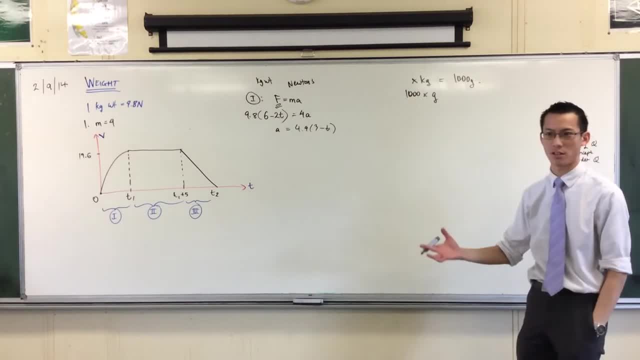 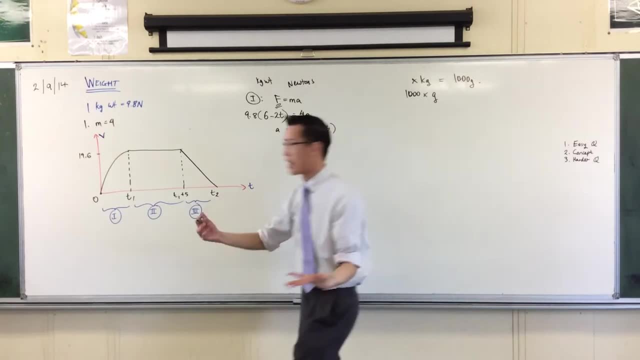 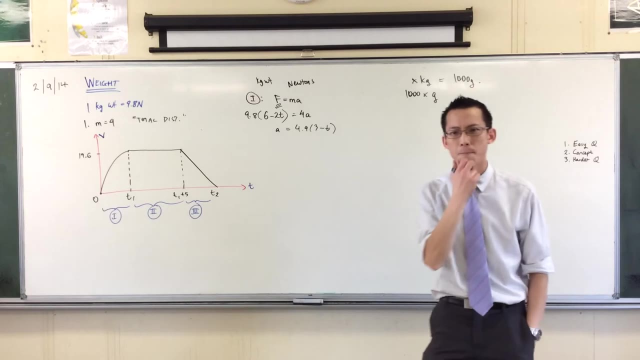 Now, where am I trying to go? Now I have an acceleration equation and it's in terms of time. Remember, we have all of these fancy ways of writing acceleration, Right. The question I'm trying to answer is total distance, So what do you think is the most direct path to get there? 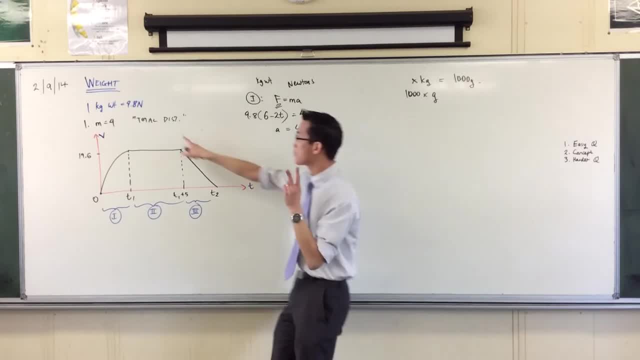 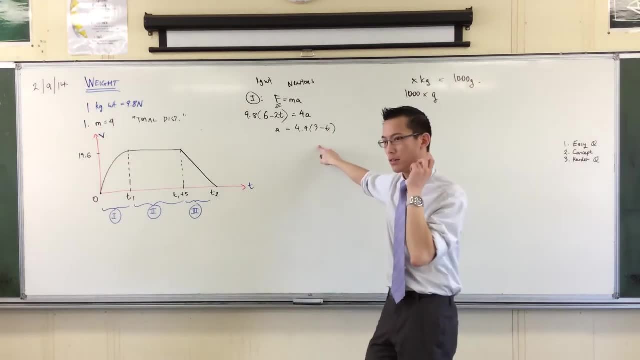 Hmm, Now I've got two pieces of information Where I'm going Like, this is what I'm trying to find And what I've got it in terms of Okay, Now it's in terms of time. So, therefore, if I'm going to integrate, I have to integrate with respect to time. 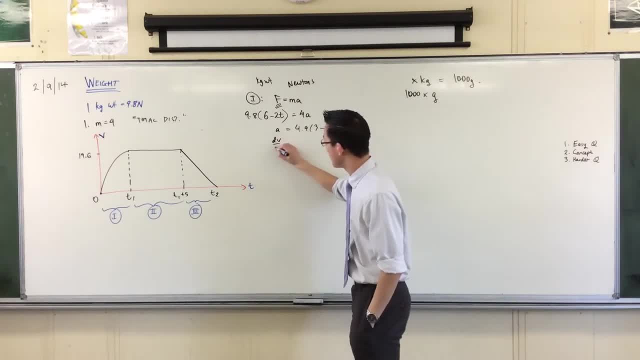 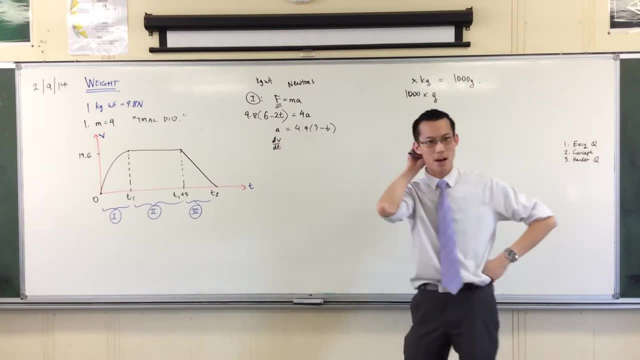 So therefore, that leads me to think probably dv dt is the most helpful way to say it. Okay, If I'd written like, say, v dv dx. I'd then be like, oh okay, I'm kind of stuck because 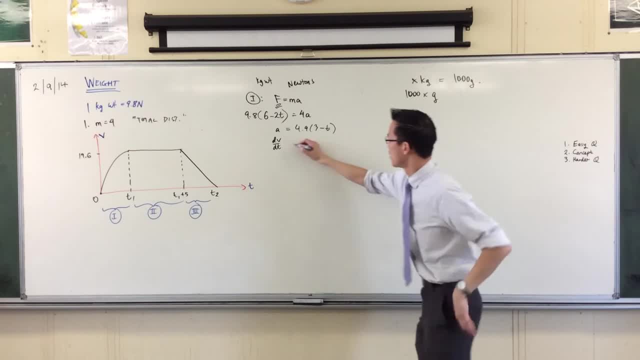 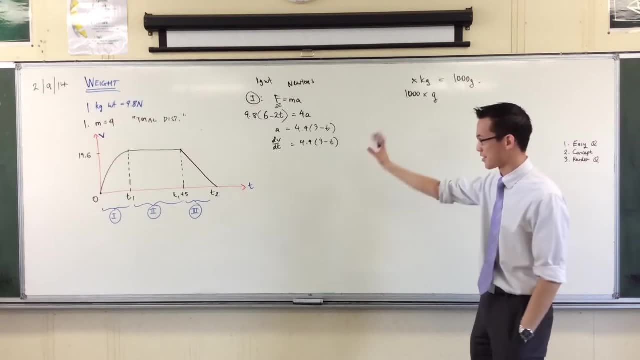 I don't have other things in terms of x to go with that, Okay. So there we go. I've got this. Okay Now, because other parts of the proof of this are going to take a little while I'm going. 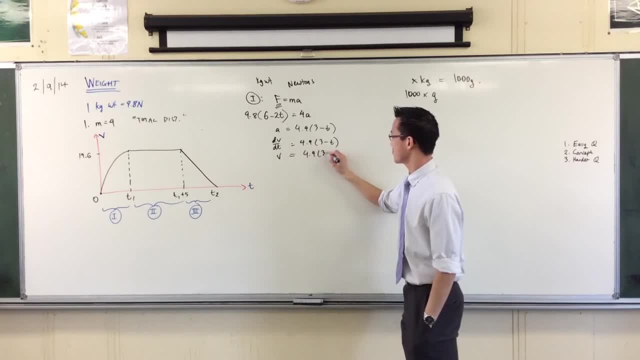 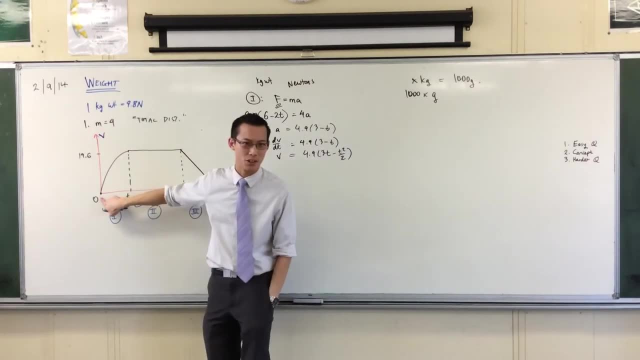 to cheat a little bit And I'm just going to go straight to here. I know there's a constant, but you can see why it's zero. Right, Can you see why it's zero? It's because I have this value. 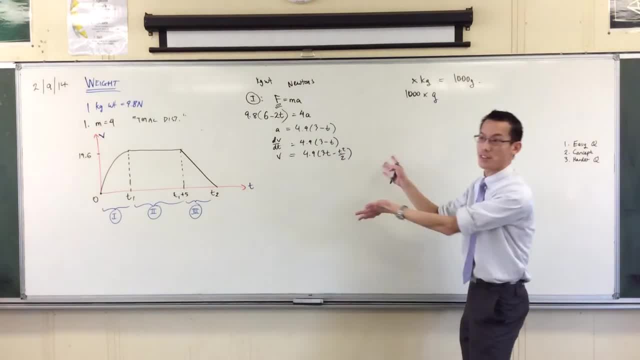 Right, So you can go ahead and you can evaluate it. Not that big a deal. That's the velocity equation you're going to end with. What do I do with this? Where do I go from here? Remember, what am I trying to do? 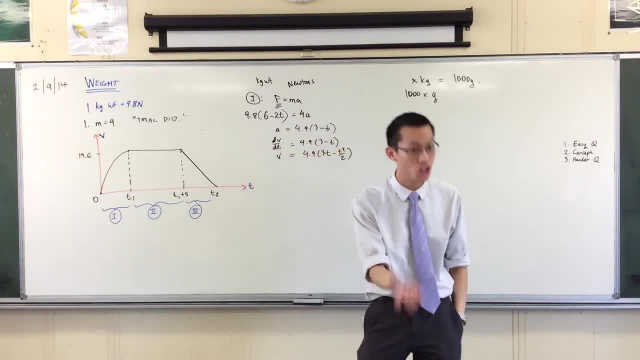 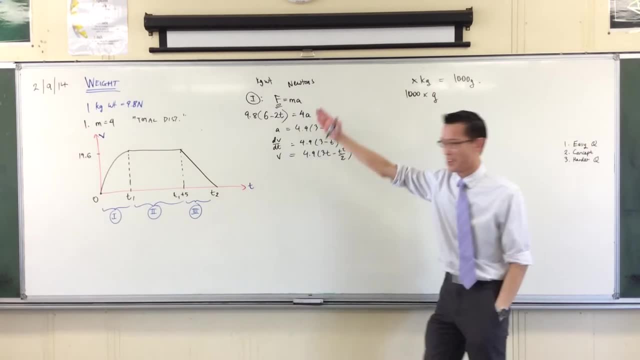 I've chopped this thing into three different parts of the journey, Right? So in order to work out how far I've gone in this part of the journey, well, you kind of need to know how long that part of the journey lasts. 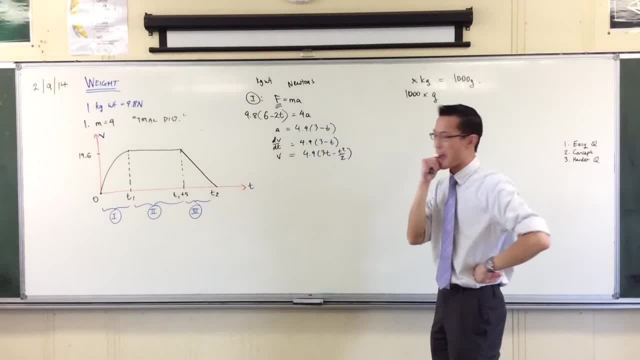 Does that make sense? So how do I know? How will I work out when the journey this part, section one, how will I know when it ends Good? The question says: The question says when the particle reaches a speed of 19.6.. 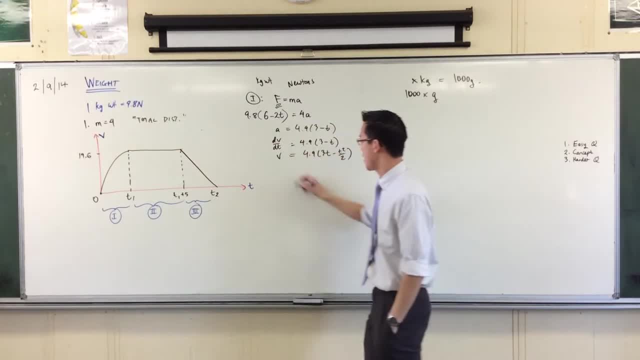 And you can read it off your graph: Right? So I can say Right. Well, okay, Let's put that in Right. 19.6.. This is what I'm trying to solve now. I'll get a time. 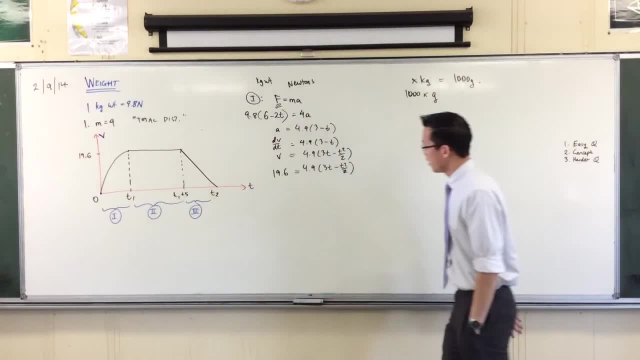 Namely, I'll get time one. Right, That's what I'm going to get: 19.6 divided by 4.9, very conveniently, is four. Okay, So now I've got three t minus t squared on two. 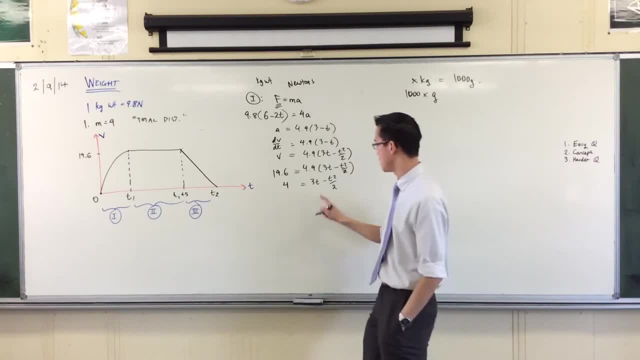 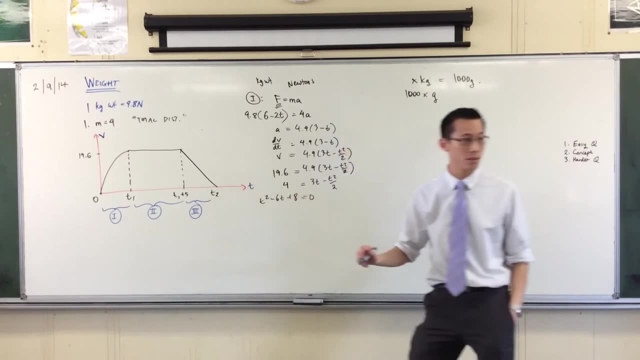 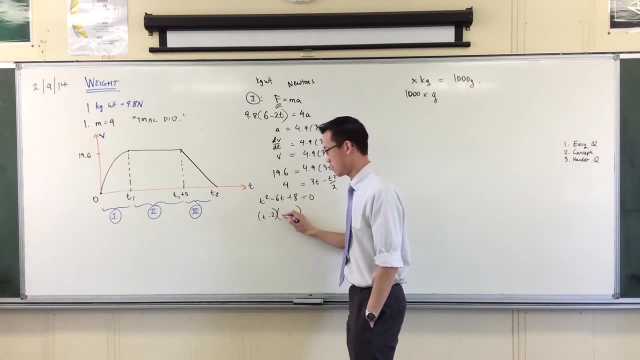 Rearranging. tidying up to make the quadratic a bit easier to solve, I guess I'll multiply by two. T squared minus 16 plus eight equals zero. Okay, You factorise and you get what: T minus two, T minus four. 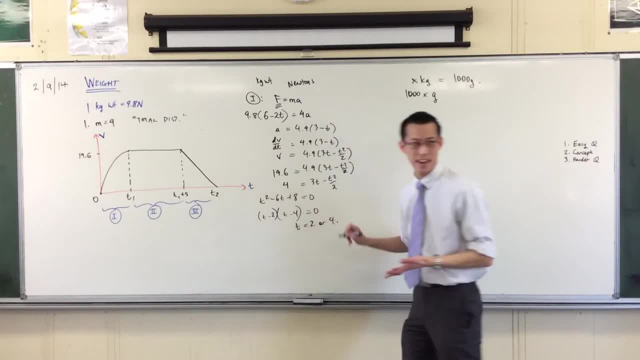 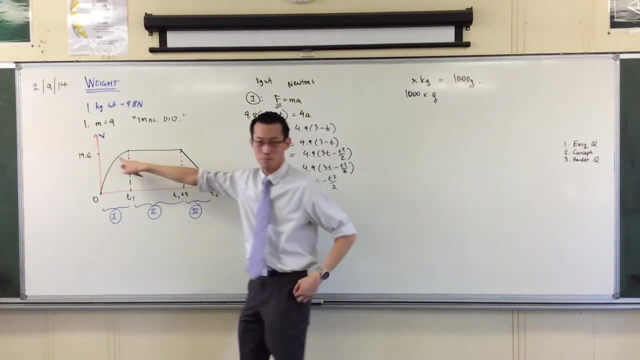 Okay, So you've got two sensible solutions. Okay, But of course, the one that you're after is this one: Right, As soon as you hit that, you've hit the requisite speed. Okay, Is that alright? I guess what that would mean is, if it hadn't have stopped, it would have kept on increasing. 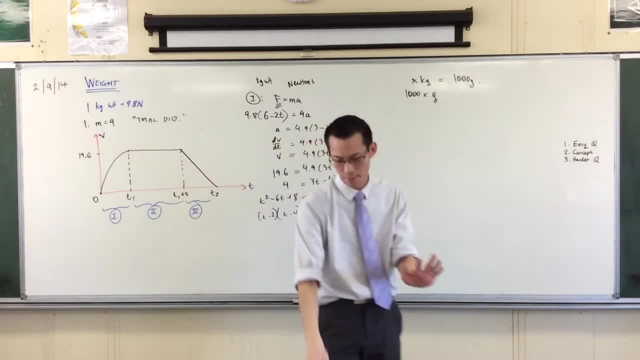 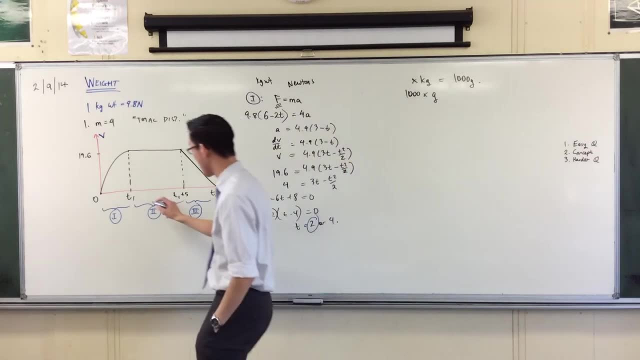 and then come back down to 19.6.. But we're not interested in that part. Okay, So I say okay. t equals two is the valuable thing, So that's really good. I've worked out what this time is. 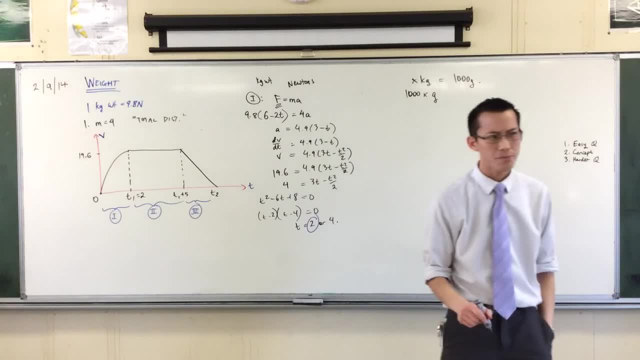 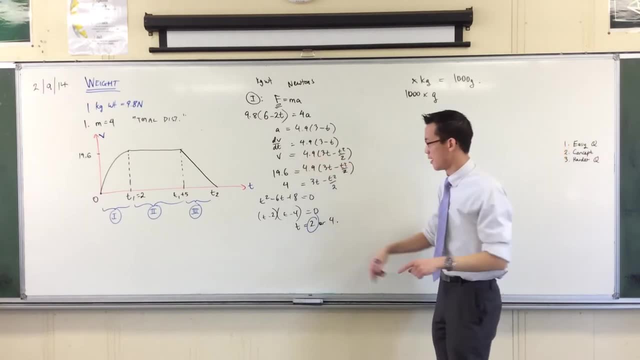 What do I do with it? What I'm trying to find is displacement. I'm only on velocity, So I'm going to climb up the ladder one more time. I have a particular value in mind. I want to go from zero to two, so it's a definite integral. 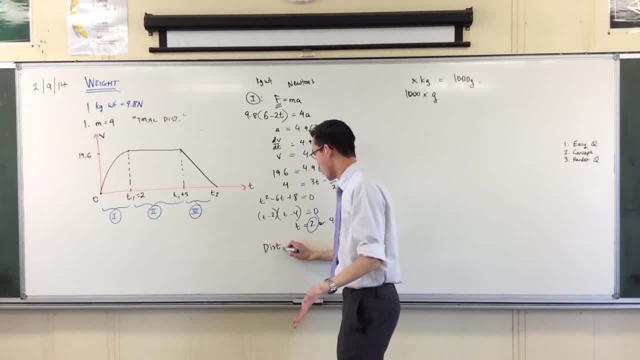 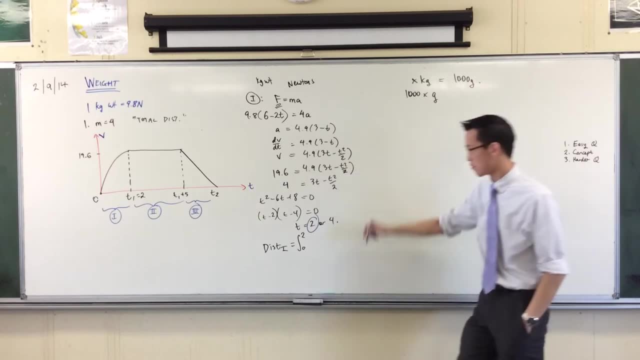 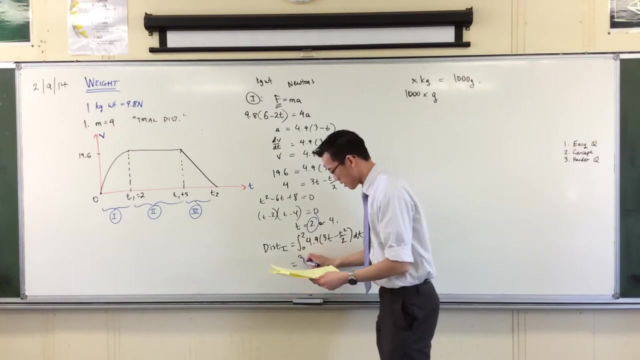 Right. The distance for section one is going to be from nought to two of v dt Right. Okay, So no big deal. You can crunch through that. I think the answer you should come up with is this: Once you integrate properly, get the right primitive and chuck in your upper and lower. 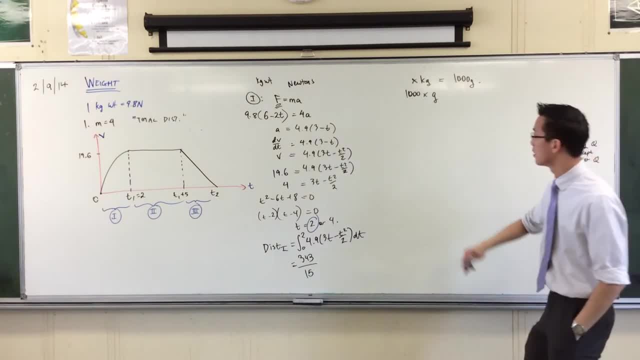 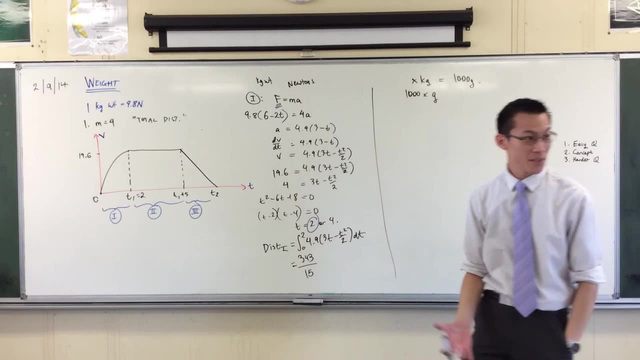 boundaries, Okay, And you can go ahead and you can verify that. So now what? What do I do at this point? Well, I only did the first section of the journey, Right, The first two seconds. Now I have to work out the rest of it. 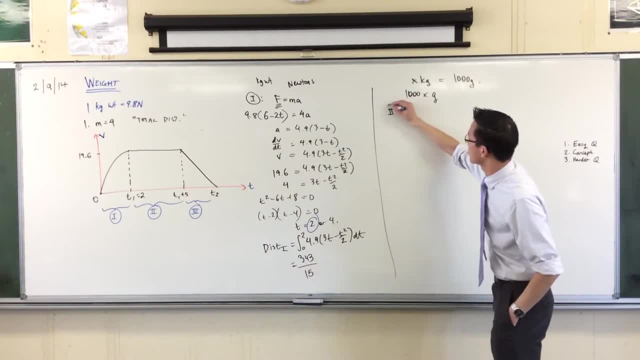 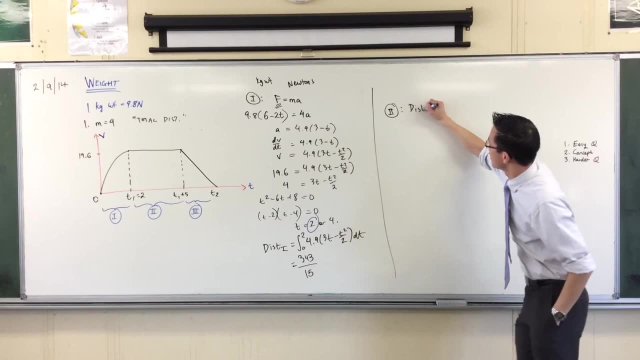 Okay, So I can say: well, section two, as it happens, is really easy. It's kind of trivial, Right Distance Distance. The distance for this part of the journey, Distance, at least as far as I remember, is speed times time. 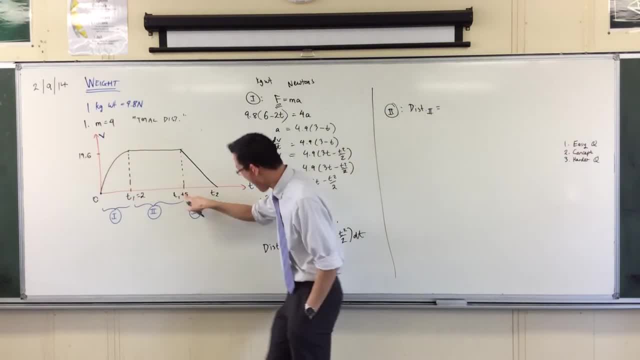 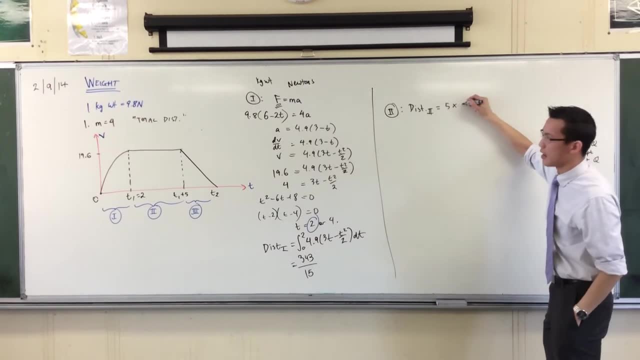 Right Speed times time. Five seconds is how long he's going for that constant part of the journey. Okay, So five times. what did I say? Nineteen, point six: Okay, What is that It's like? oh, I don't know. 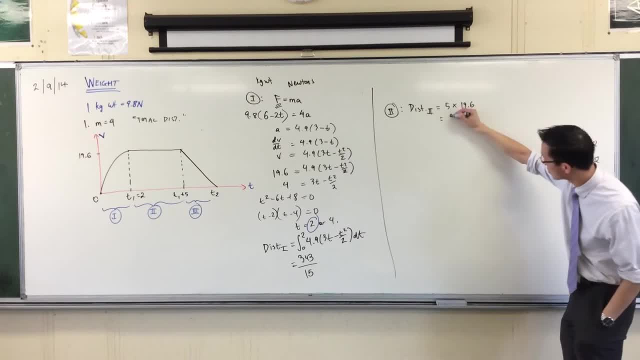 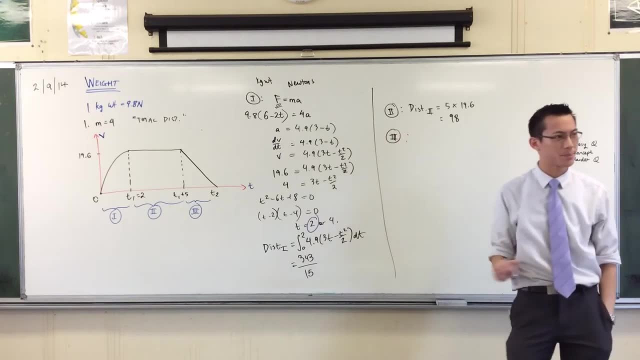 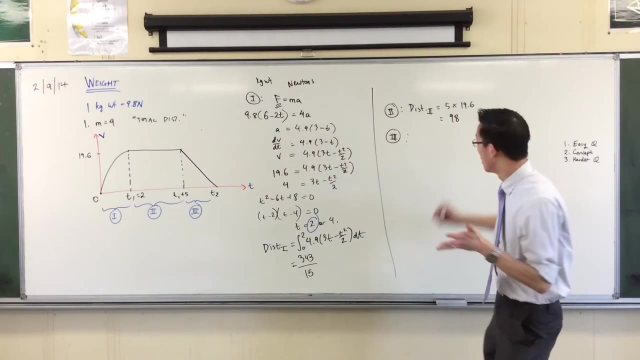 Five times nineteen is ninety-five. Five times point six: ninety-eight. I think That part's easy. Last part, Okay. Now this part is very similar to what we had here. Right Again, they give you a force equation. 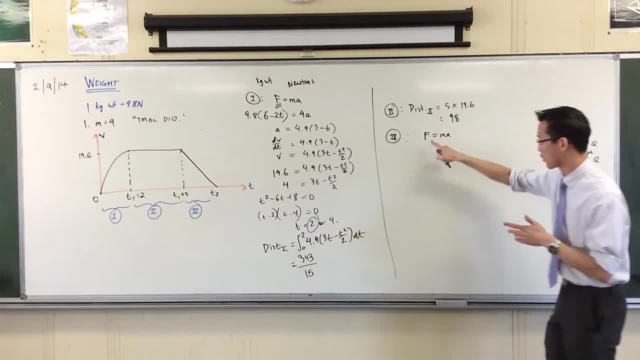 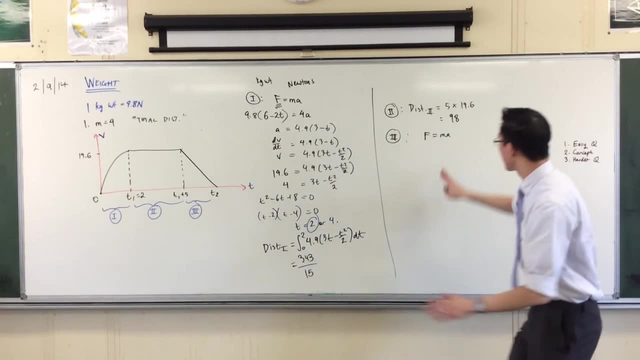 So I'm still going to have F equals MA, even though it's a different force. Okay, The equation they give you- let's see where am I up to- is that it's a constant force of five kilograms, Five kilograms weight. 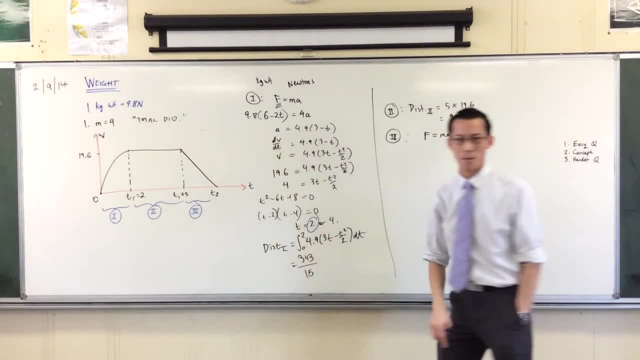 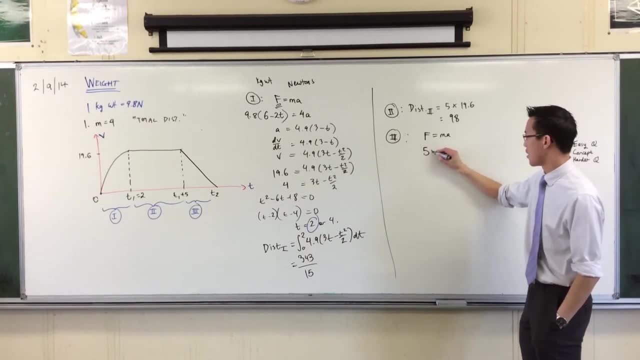 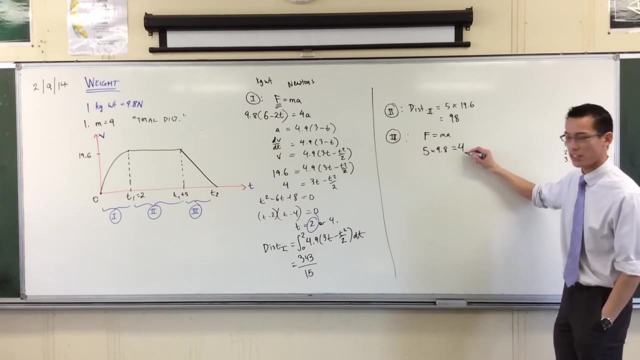 Five kilograms weight. Now pause for a second and look up Five kilograms weight. It's five, It's nine point, eight times bigger. What's the mass? Still four. That hasn't changed. And then there's acceleration Right. 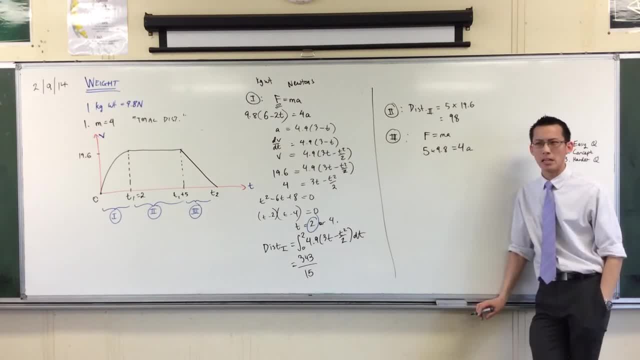 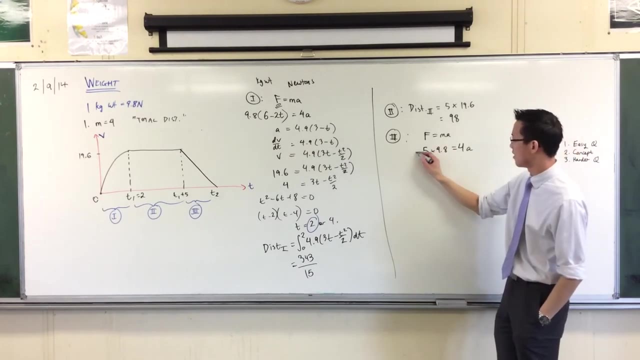 I'm missing something. What am I missing? Look carefully, Read the question again, if you have to. What's wrong with this line? Something is drastically wrong. Aha, Why. Why should there be a negative? It's very common sense when you think about it. 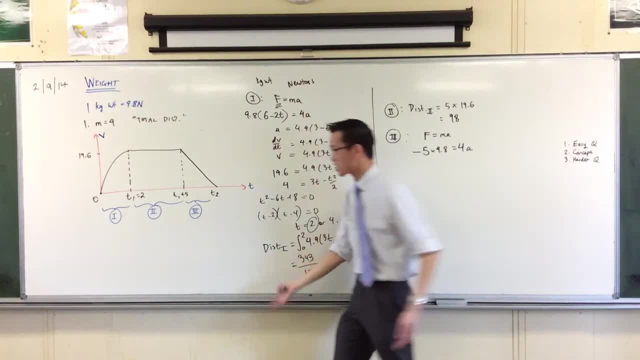 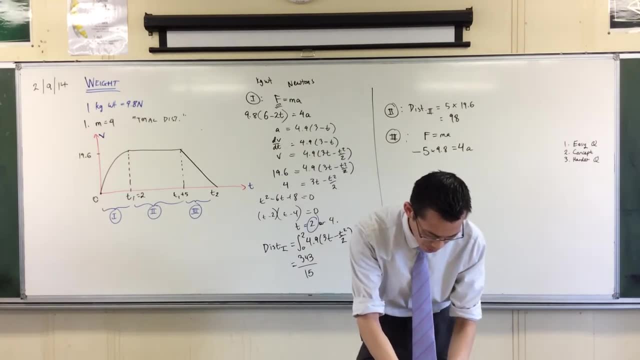 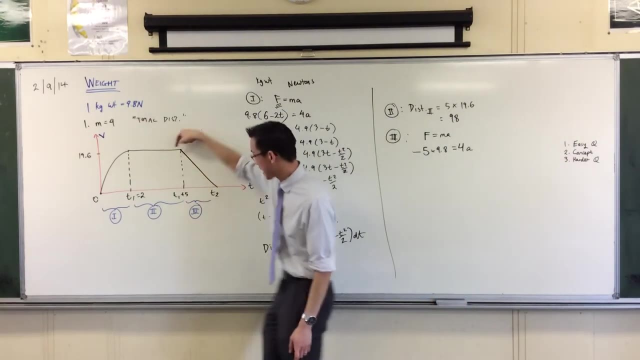 What's this force doing? What's this force doing? It's speeding you up, Right. It's speeding you up So positive direction, Right, Because at that end point it's then brought to rest. So, whatever this force is doing, it's got to get it away from being at a constant speed. 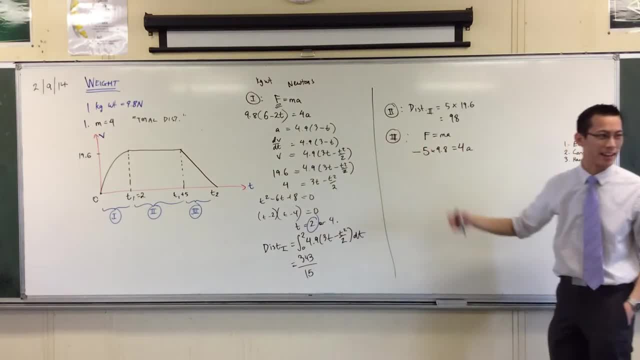 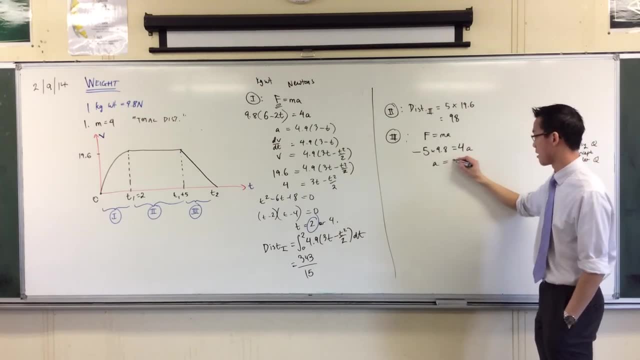 get the velocity back down to zero. Okay. So hence a negative. Right From there you can solve. Okay, I think that's 29, if I remember it right. So you've got that acceleration. Okay, Now you have to be a little more cautious, because when you integrate, 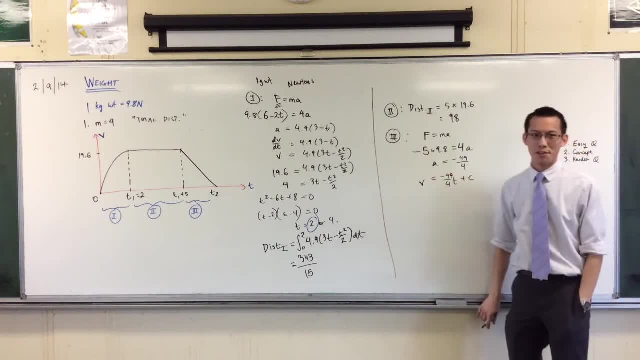 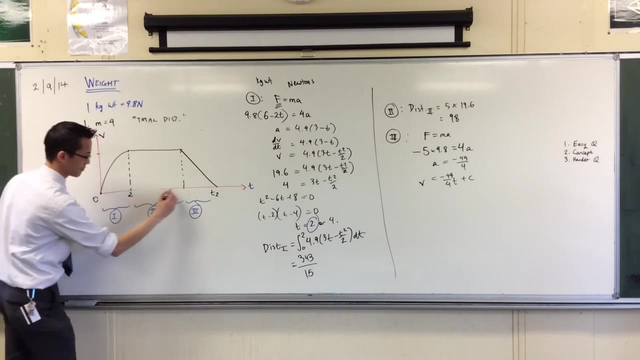 you've got to be a little more cautious. You better believe that constant's not zero, Right? How do I work out what the constant is? I just gave you a clue in case you hadn't noticed. How do I work out the constant? 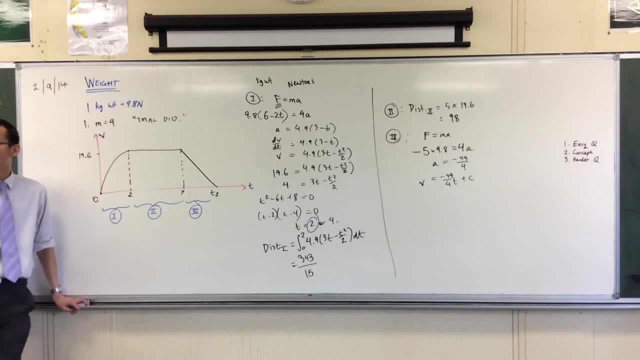 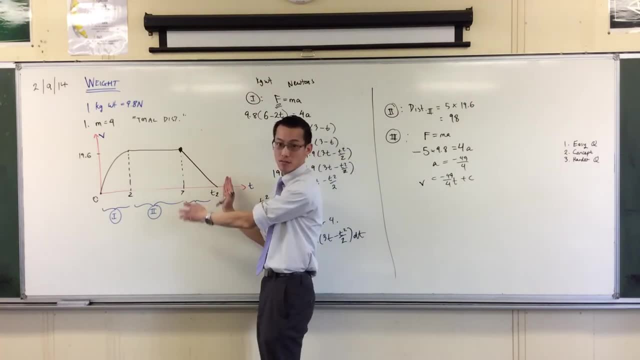 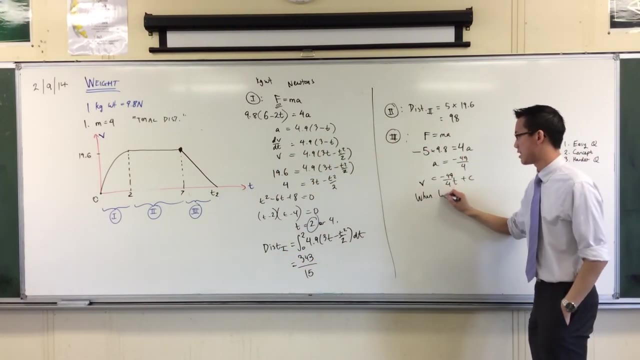 Because it's not zero. Ah, good, I have a condition: That one, Right, It has to be this one because it's got to be in section portion three, Right, That's when this rule takes over. Okay, So I can say when t equals seven. 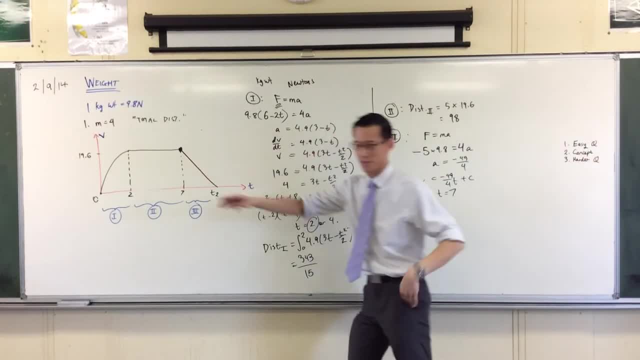 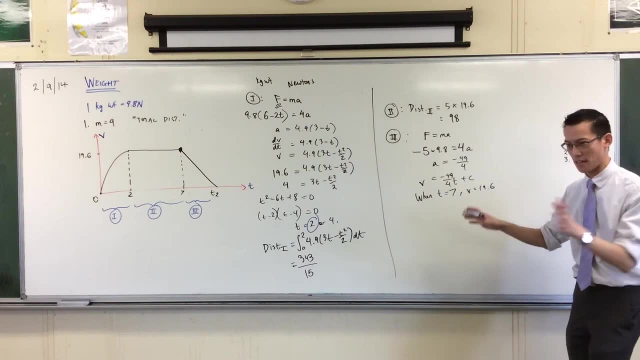 Right, When t equals seven. this point there after the first journey. five more seconds, then the velocity is 19.6.. Okay, It turns out a bit gross. The numbers aren't very friendly, but you work out the constant. 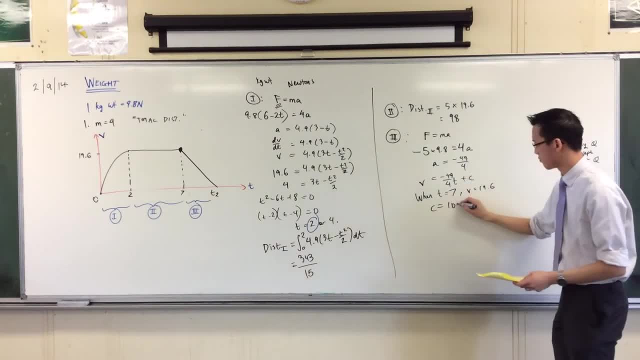 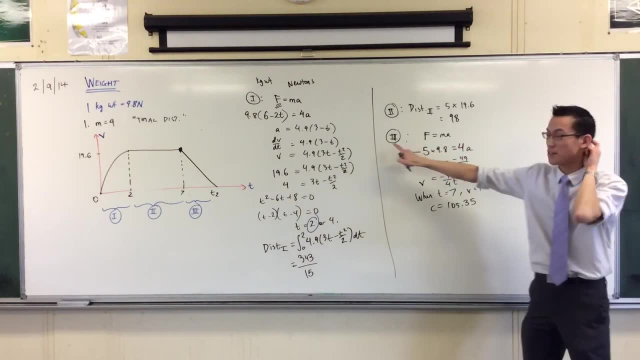 And I think you should end up with this. Yuck, but at least it's not a repeating decimal, Okay. So now I have the velocity equation for the last part of the journey. Okay, The velocity equation is this Plus: 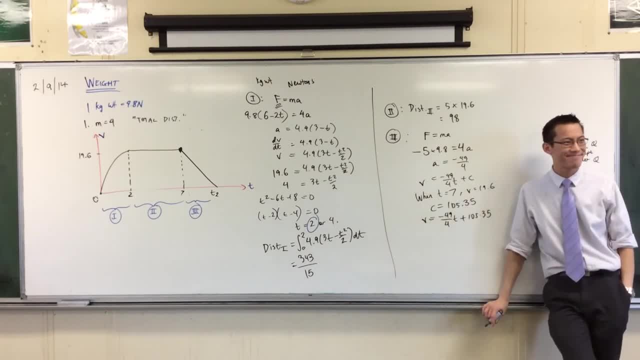 Okay, What do I do with this thing? What do I do with it? Think back to how I dealt with section one. I want to get towards integration, but I don't know what to integrate between. I know where to start, Right. 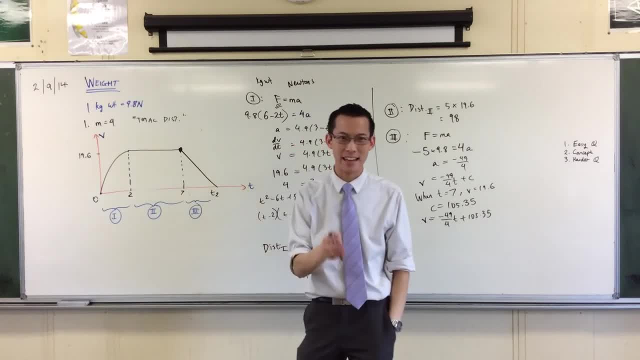 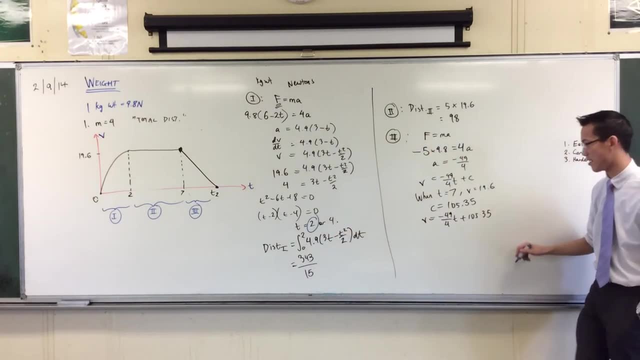 But I don't know what this final end time is. But it's not that hard, is it? It's just like the question we just looked at. You've got to work out when v equals zero. Okay, So you're going to solve for v equals zero here. 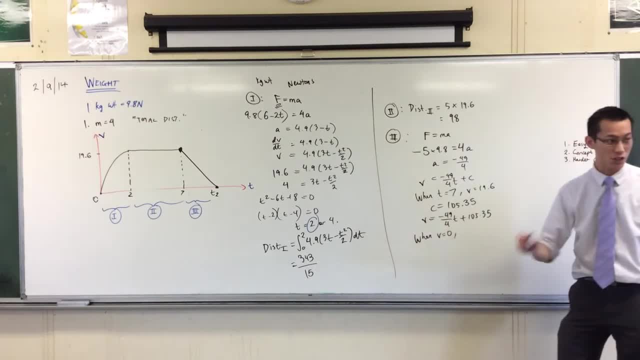 Okay, When v equals zero, You go ahead. You crunch the numbers. I'm pretty sure it's 8.6.. Okay, Double check it, Confirm it. But this is not the hard part of the question. This is just the crunching part of the question. 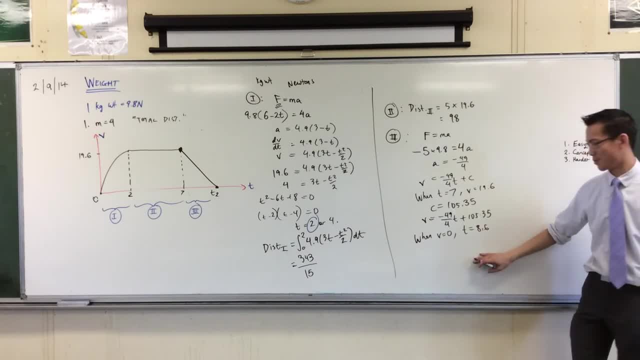 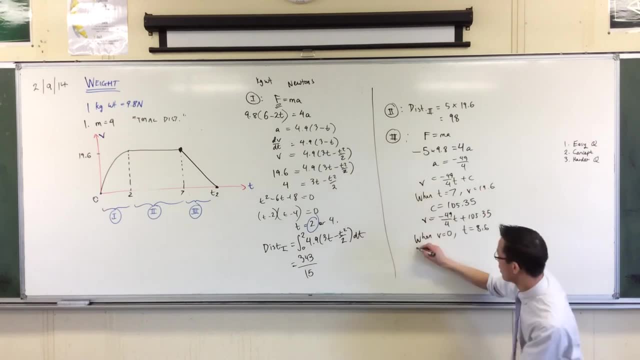 Okay, What do I do with this value? No, seriously, What do I do with this value? I have to integrate again, Just like I did here. Okay, So distance three: It's going to be the integral from where to where.